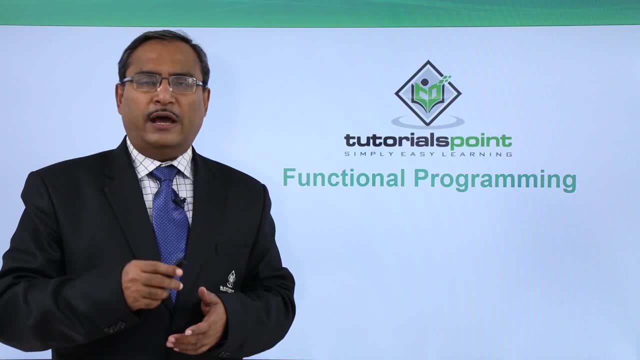 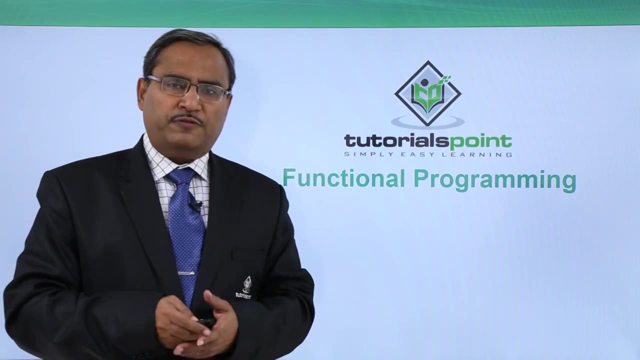 of the procedural programming. if you also pass the same value for multiple number of times, then the procedure may return different values on its execution. So let us go for further detailing on it. So functional programming is style of programming language which uses 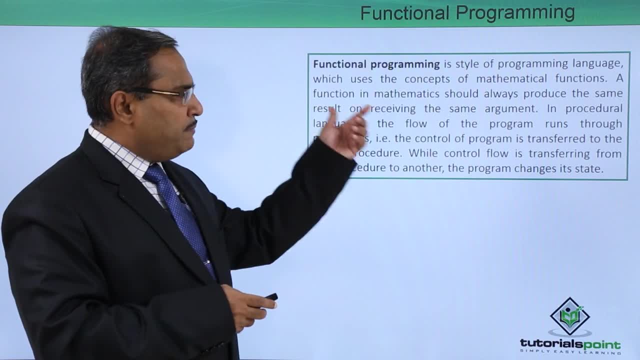 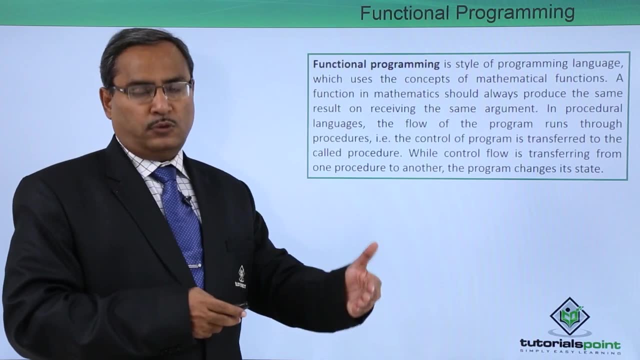 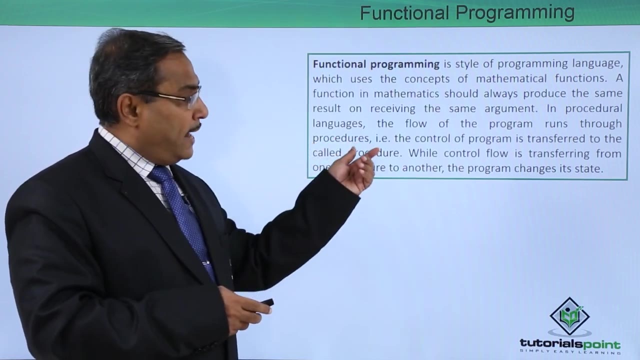 the concept of mathematical functions. A function in mathematics should always produce the same result on receiving the same argument. So argument means here we are considering as the input argument And in procedural languages the flow of the program runs through the procedure and that is the control of the procedure. 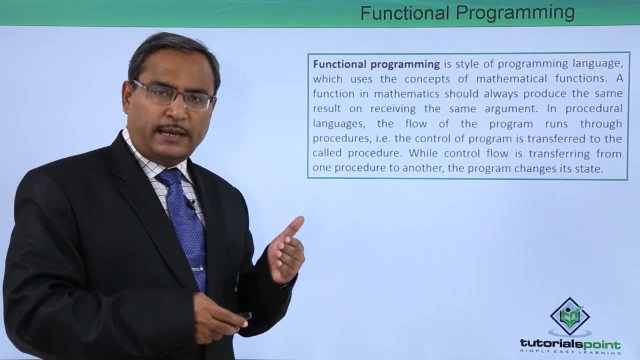 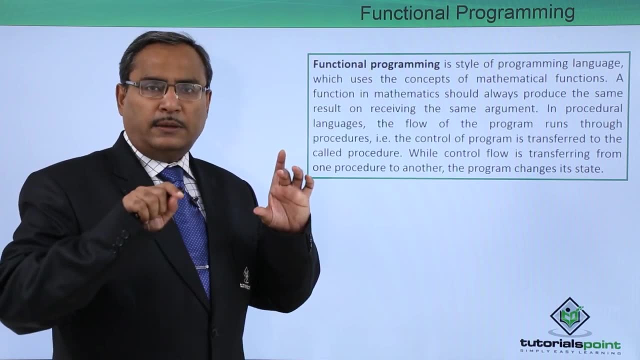 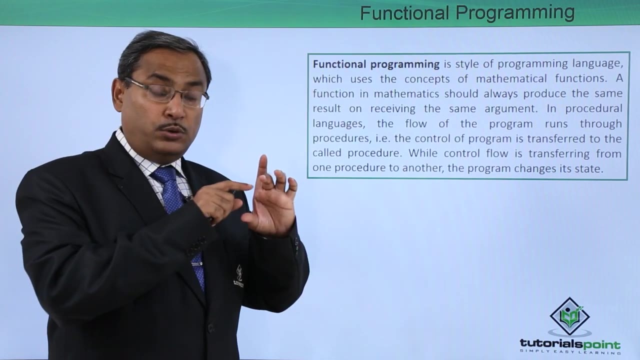 The flow of the program is transferred to the called procedure. So whenever a procedure will be called from a certain code, then the control will be transferred to the respective procedure body and there the procedure will get executed. After completion of the procedure execution, the control will come back to that very line, which is just after the line of 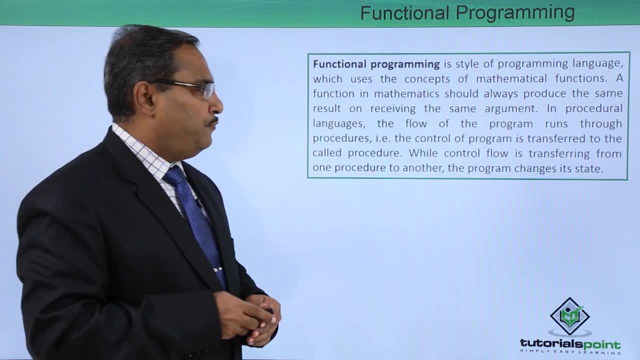 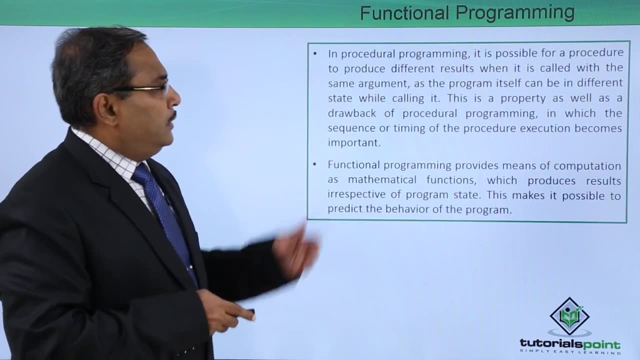 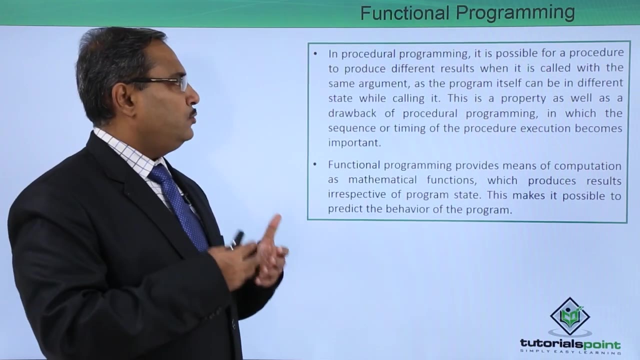 the calling procedure statement. While control flow is transferred from one procedure to another, the program changes its state. In procedural programming, it is possible for procedure to produce different results when it is called with the same argument, as the problem itself can be in different state. 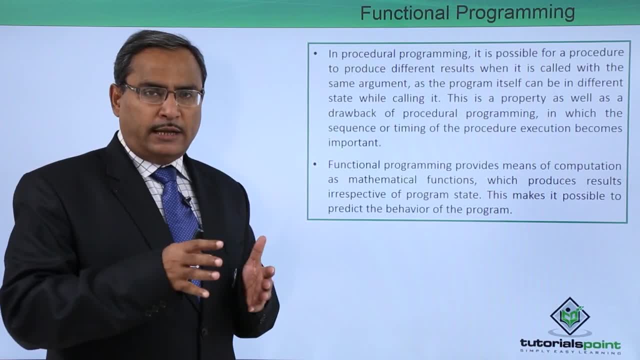 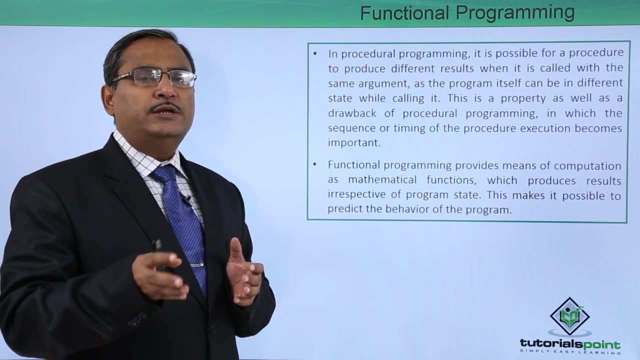 while calling it. So that is why it is not mandatory that, in case of a procedure, whenever you are passing same arguments for multiple number of times, the procedure will return you the same value because, depending upon the state of your program, the procedure may. 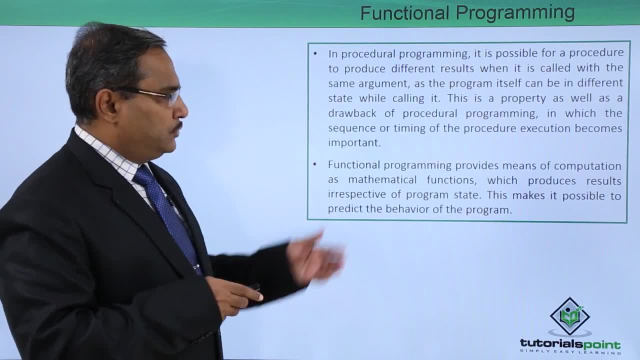 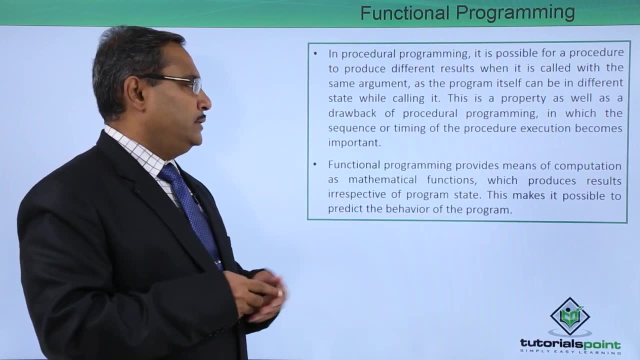 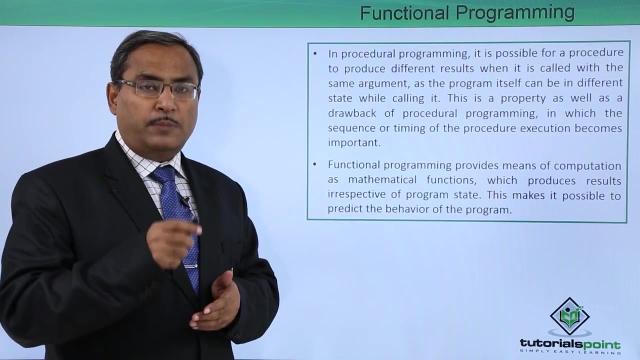 return different values as outcome. So this is property. this is a property, as well as a drawback, of procedural programming, in which the sequence of or timing of the procedure execution becomes very important and the output, the outcome of the procedure, depends upon the state of the program. 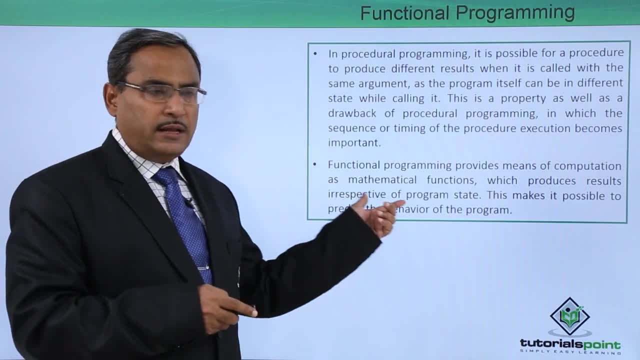 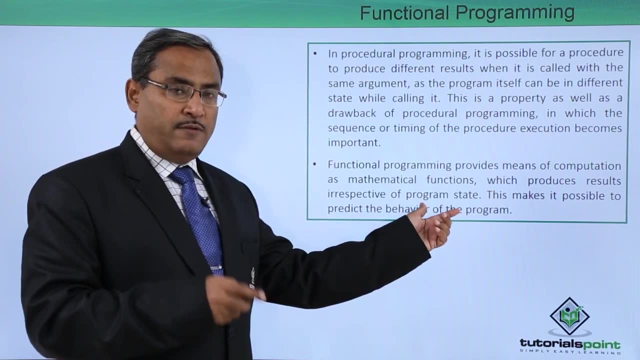 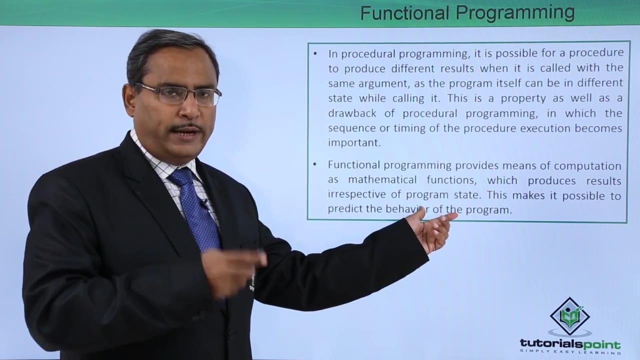 Functional programming provides means of computational as mathematical functions, which produces results irrespective of program state. We discussed this, This one earlier. for the same inputs we pass for the multiple number of times the functional in the. in case of functional programming will be going to get the same output irrespective. 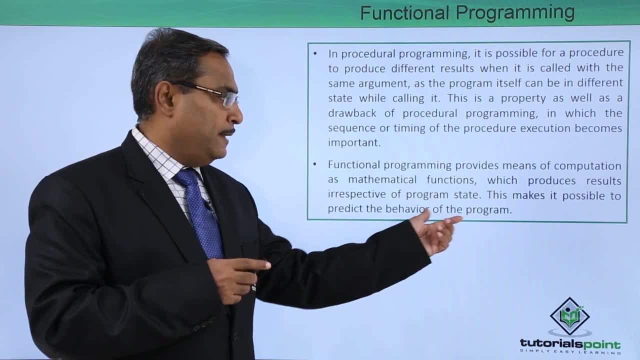 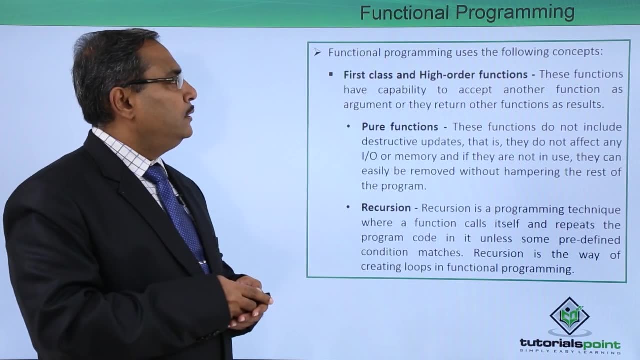 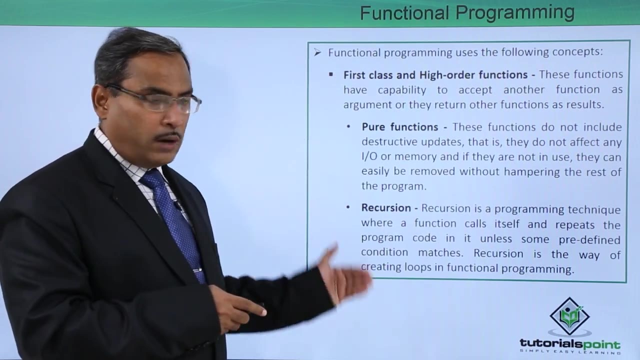 of the current state of the program, irrespective of the timing. This makes it possible to predict the behavior of the program. Next one is a functional programming uses the following concepts. So what are the concept they are using? Let us go through them one by one. 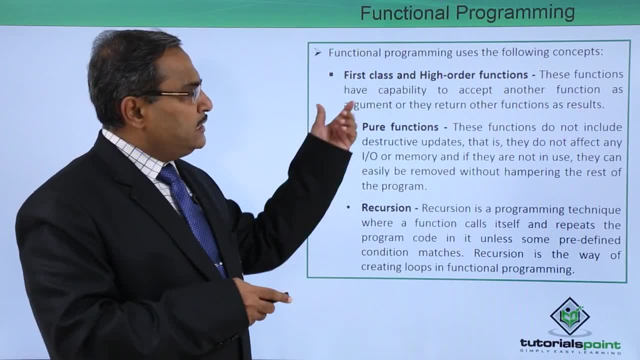 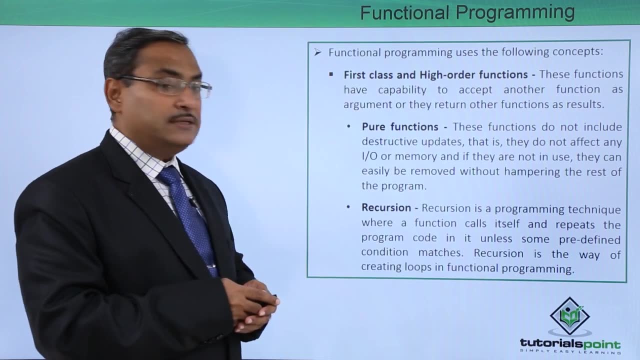 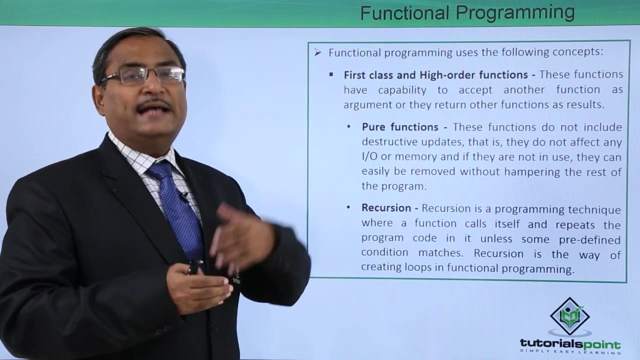 So first class and high order functions. So these functions have capability to accept another function as argument or they return other functions as result. So this is very interesting: A function will take another function name as input argument and as a result also one function can return another function as the output. 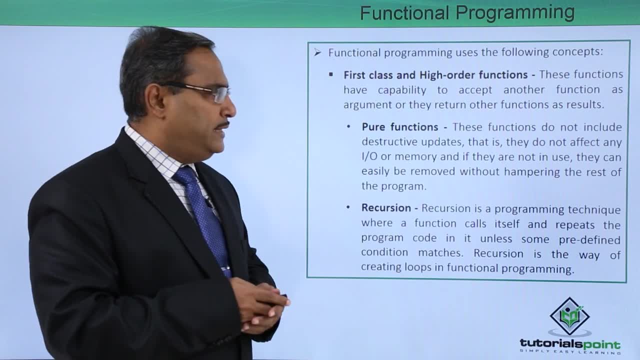 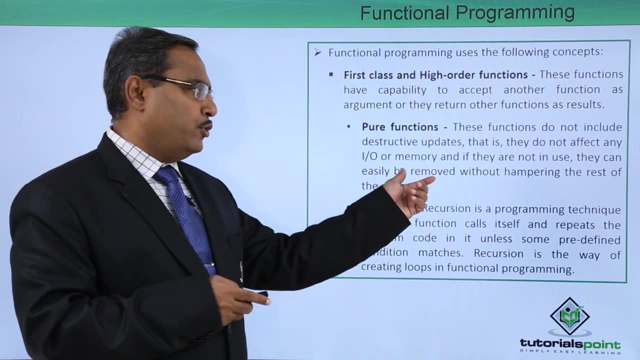 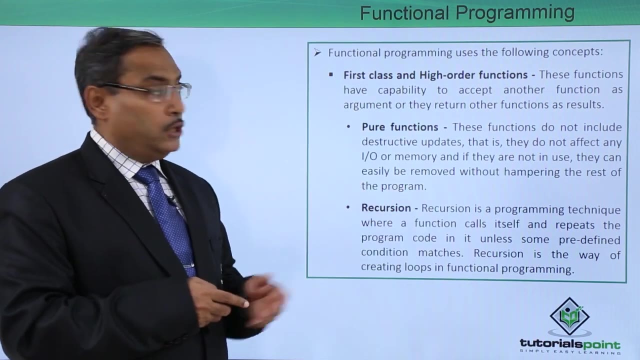 So let us discuss this pure function at first. So these functions do not include destructive updates, That is, they do not affect any I O or memory, and if they are not in use they can easily be removed without hampering the rest of the program. So here there is. there will be no. 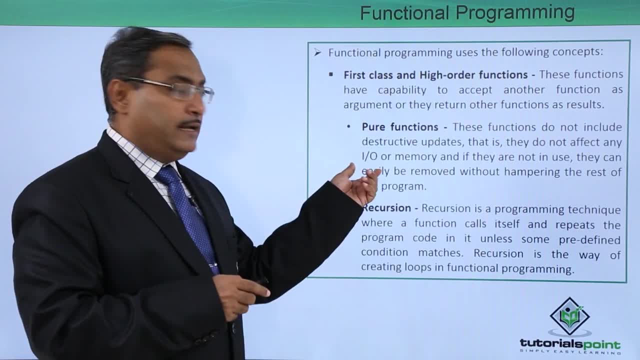 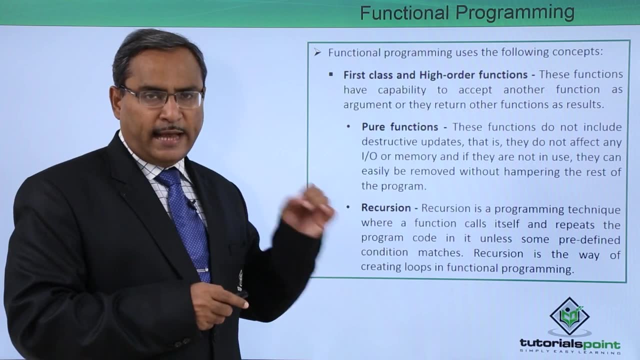 destructive updates, So it is not actually affecting any memory location or any I O. and when this pure functions are not getting called or not getting accessed or not getting executed, you can easily remove them without disturbing the system. So next one is our recursion. 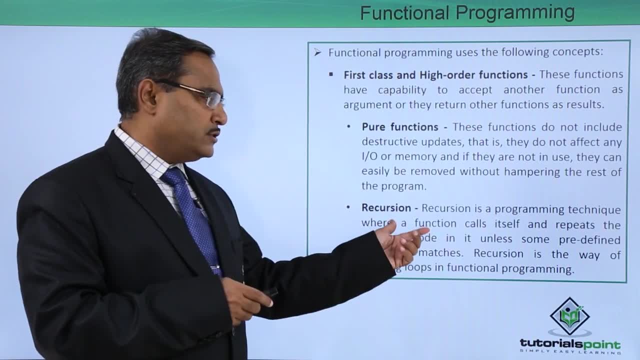 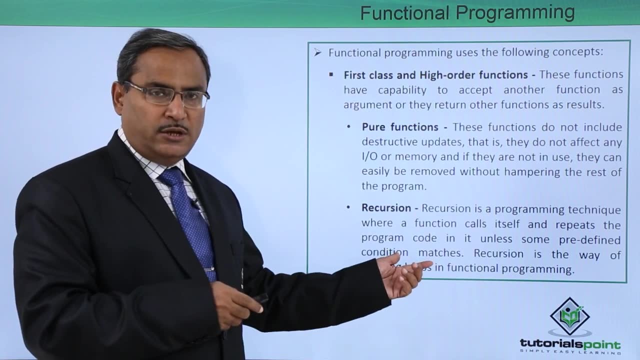 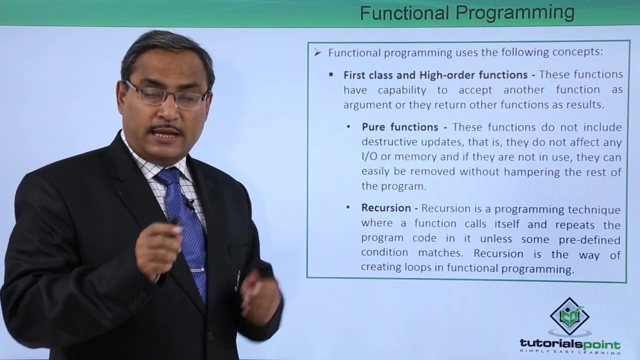 A recursion. Recursion is a programming technique where a function calls itself repeats the program code in it, unless some predefined condition matches. We know that in case of recursive algorithm there will be some base case, So for certain inputs, outputs will be known to us and where this recursion will terminate and recursive. 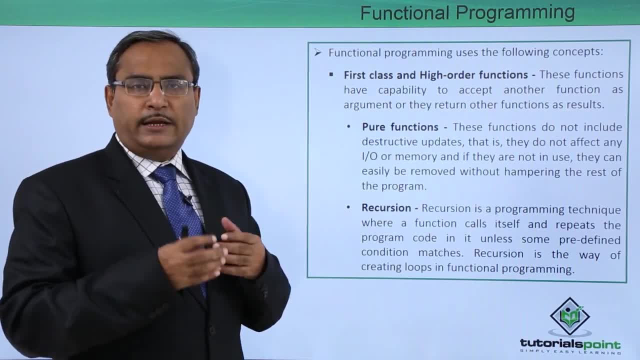 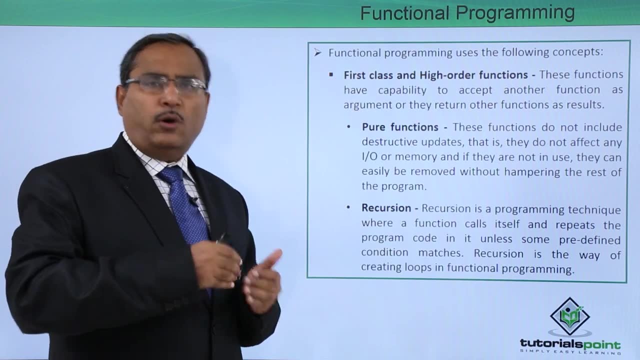 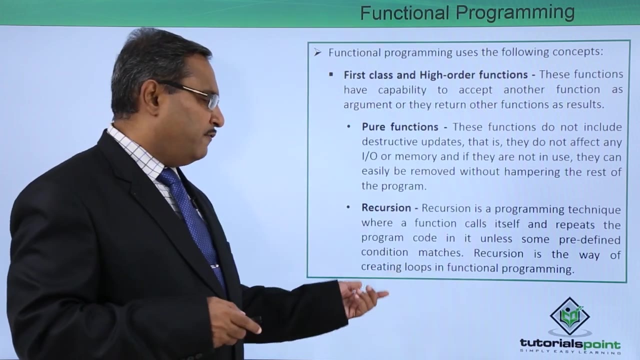 algorithm will have a capability to call itself either directly or indirectly. Direct calling means the recursive call will be within the function body itself. Indirect calling means it will be calling another function. that function in turn will be calling the parent one. So recursion is the way of creating loops in functional programming. 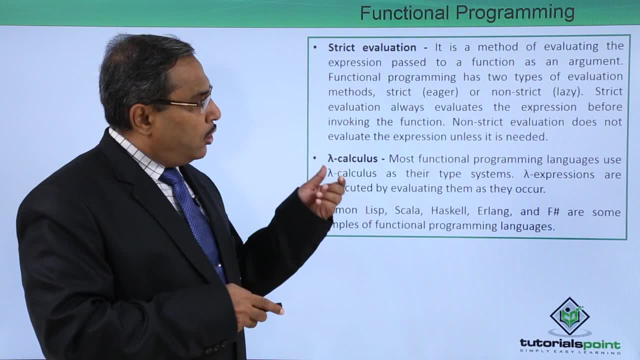 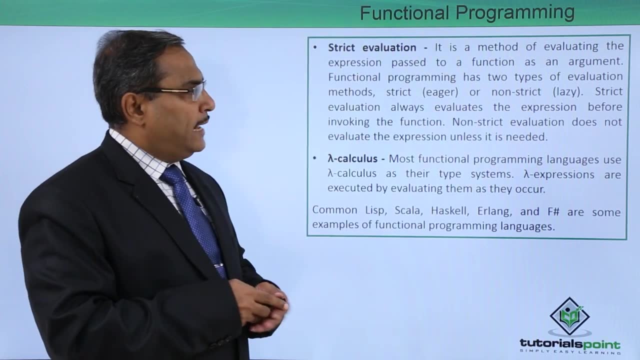 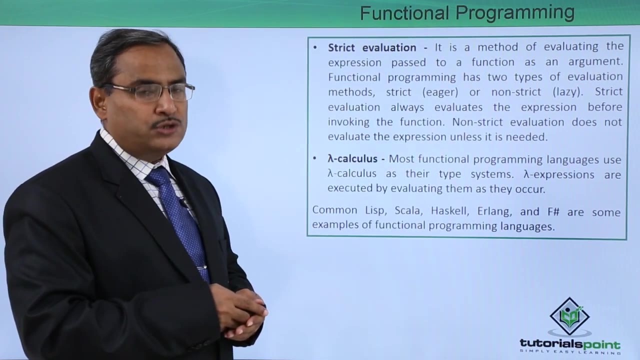 Next one is the strict evaluation. It is a method of evaluating the expression passed to a function as a argument. Functional programming has two types of evaluation methods. one is the strict, that is the eager. another one is a non strict that is known also as the.